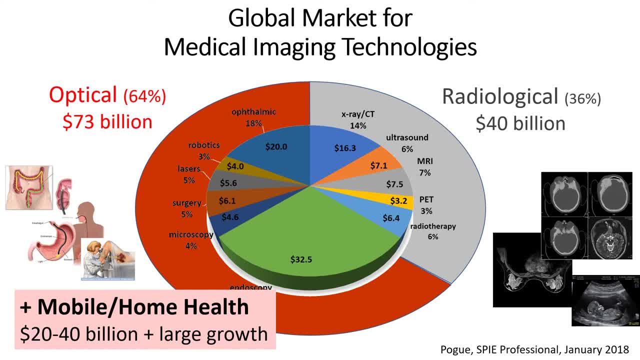 of the radiological field And I think this comes as a surprise to many people. And then you add in the growth in double-digit growth in home and mobile health devices, which are largely optical devices. They certainly aren't radiologic devices And you can easily see. 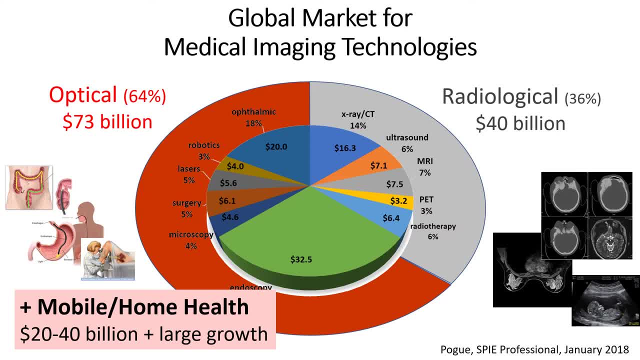 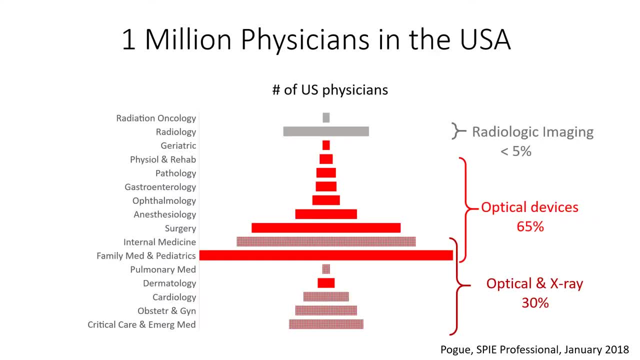 that optics is economically the largest single technology sector in medicine today. Another piece of this is: if you look at. the Another piece of this is if you look at. the Another piece of this is if you look at the unknown. For example, in the United States we have a very small physician user base. 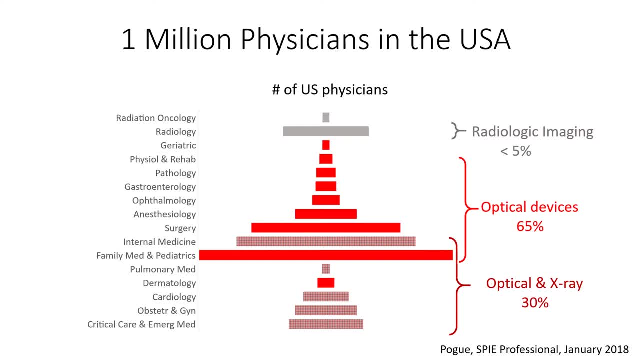 And so in the US there's about a million physicians, You know, if you look at radiation, oncology and radiology. And so in the US there's about a million physicians, You know, if you look at radiation, oncology and radiology. 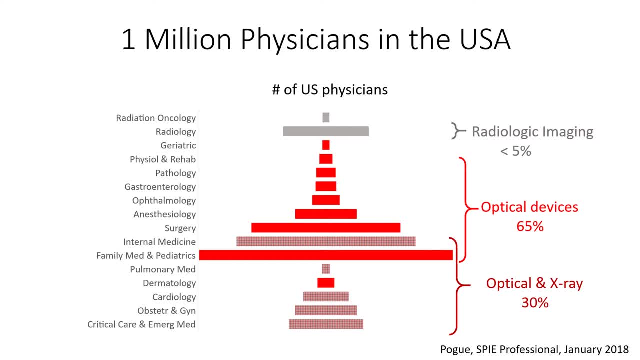 those are the hardcore radiologic users. That's only about 5% of the physicians. about 35% use about 5% of the physicians. About 65% are almost exclusively optical device people And about 30% use a little bit of both optics and x-rays, and so you can clearly see that optical devices penetrate 95% of the 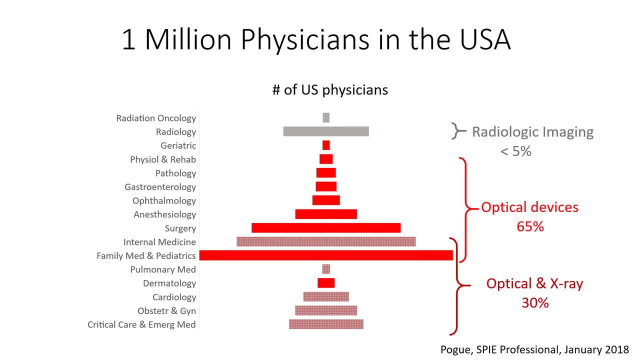 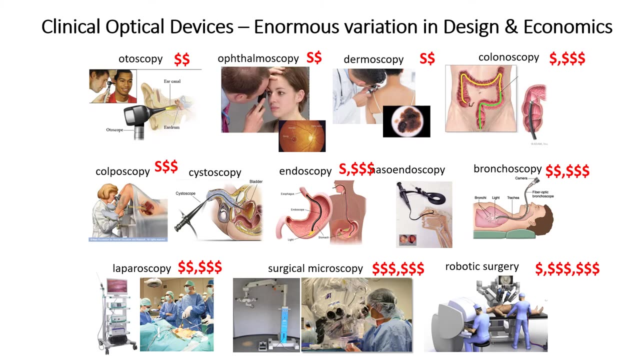 And so you can clearly see that optical devices penetrate 95% of the people- Now it's notflies that do a lot of microcosmos- 95 percent of the physicians, whereas radiologic systems really have a much smaller impact. and so again, you know the the point of care technologies tend to be optics based. the reason we don't 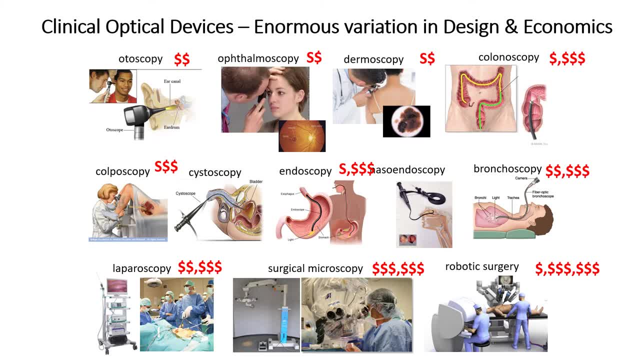 always recognize it is because of the enormous variation in different designs and economics of optical devices. you can go all the way, from a 100 otoscopy system all the way up to a close to 10 million dollar robotic surgery system and everything in between, you know. 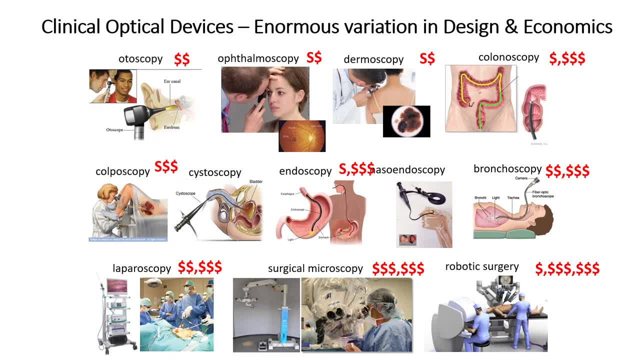 through ophthalmics, dermatology, colonoscopy, cystoscopy, colposcopy, endoscopy, bronchoscopy, up to laparoscopy and surgical microscopy. so you know the we don't always recognize this as a singular thing field, because it's permeated every field of interventional, certainly interventional. 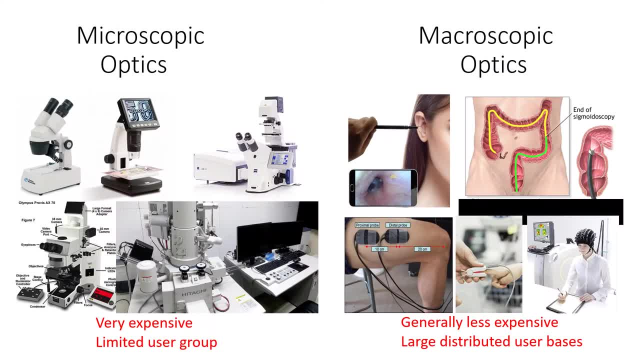 optics, interventional medicine, i should say. i think also that people often think of biomedical optics as microscopes. you know that's kind of the the obvious thing to think about. but in fact you know, if you think about it, the microscopic optics world is very small. they tend to buy very expensive microscopes, but it's a limited user group in comparison. 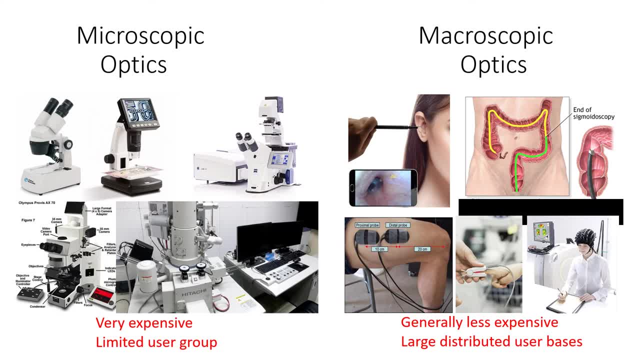 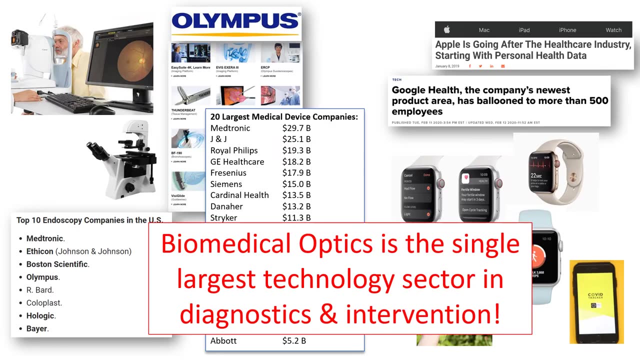 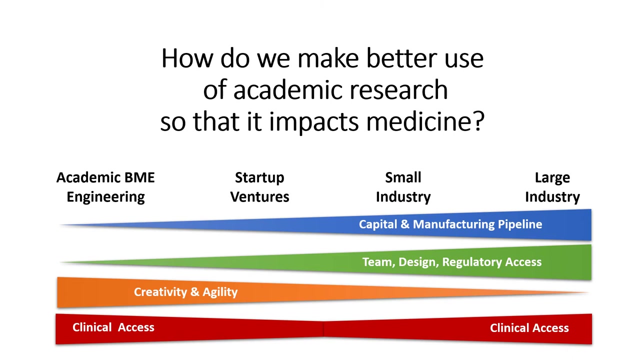 macroscopic optics, the kind that the day-to-day physician uses in sort of point-of-care medicine. these are larger type devices, highly differentiated, generally less expensive, but, you know again, permeate throughout all of medicine, you, you, and so as optical engineers, you know, I think, a lot in work, we work a lot in how. 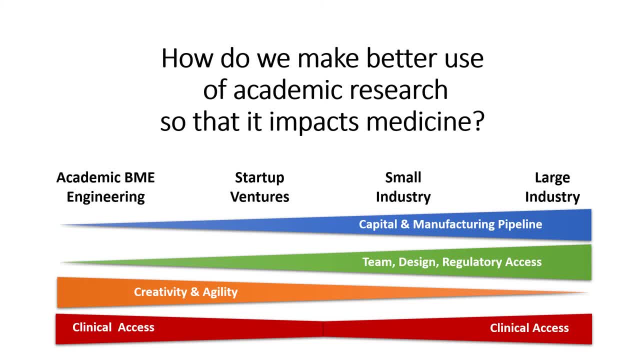 do we make better devices? and you know what can an academic do to impact medicine? and so if you think about academic biomedical engineering as compared to startup ventures, let's say, or small industry or large industry, you know there's a couple obvious things to note, right, the if you think about 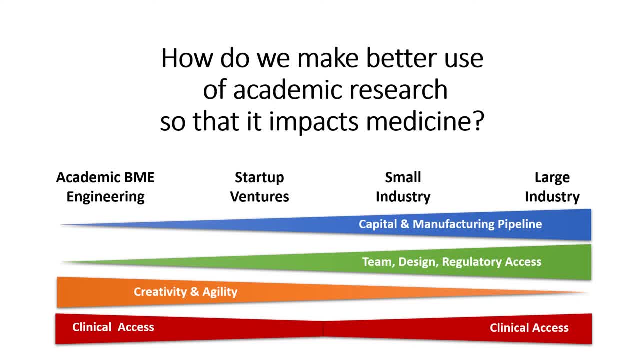 capital and manufacturing pipeline. it's much larger as you go towards the large industry. if you think about the team, the design capabilities, the regulatory access, they all get better as you go to large industry. so you know where do academics compete, where do small venture companies compete they? they compete in creativity and agility and I think they compete in 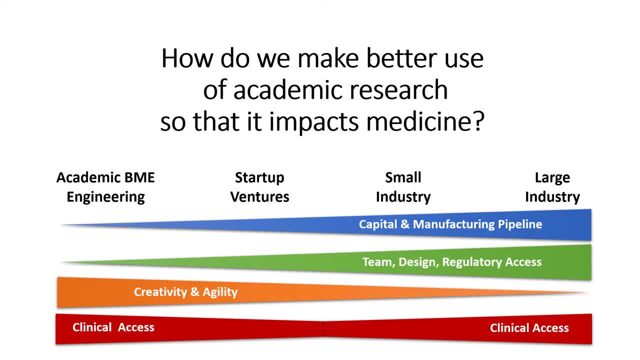 clinical access. you know, it's actually quite interesting that as you go to startup ventures or small industry, the clinical access kind of decreases a bit really. but it's the large companies that can buy their way in or it's the academics who can just collaborate for academic benefit. 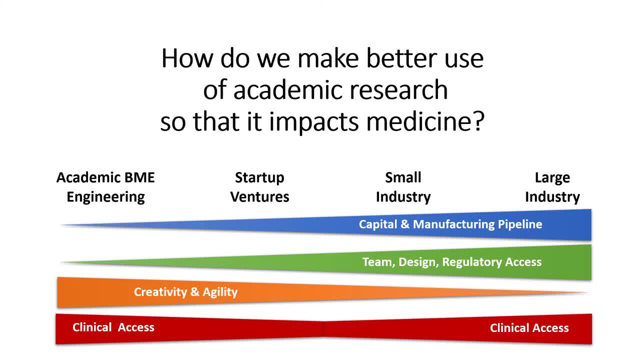 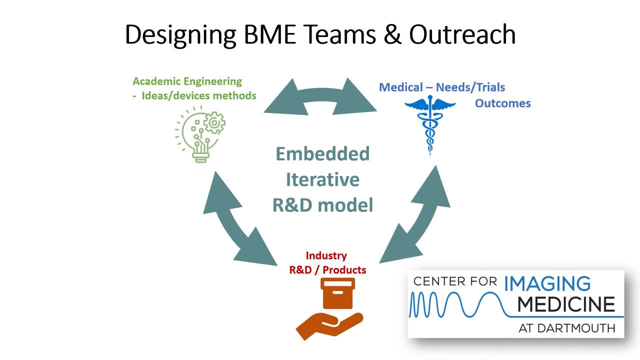 that get clinical access, and so we have to think carefully about, you know, the strengths of academic biomedical engineering being creativity and agility and direct clinical access, and so you know, this is the world that I think about. is academic engineering, being one part of it, the medical world? 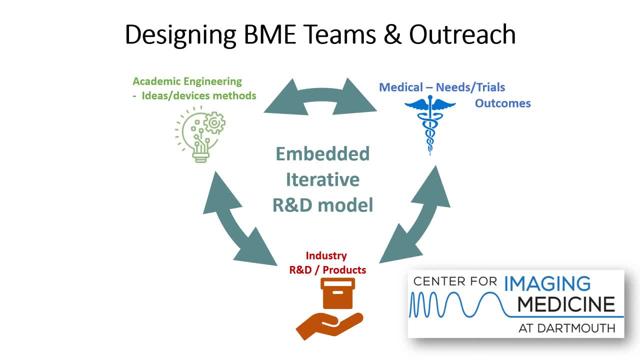 that has needs and looks at outcomes from trials being part of it. and then the industry world, where you do R&D and product development and a lot of academics just focus on pushing technology to industry or to medicine and hoping it sticks. you know a lot of companies directly put product. 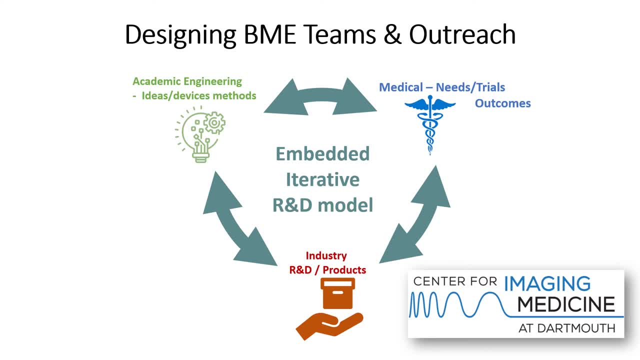 push their devices to the medical industry. a lot of medicine academics just looks at harvesting interesting technologies for medical needs. you know, I think an appropriately designed, creative biomedical engineering research group does this sort of embedded model where you embed academic engineering into the medical world and embed industry within as a part of that. 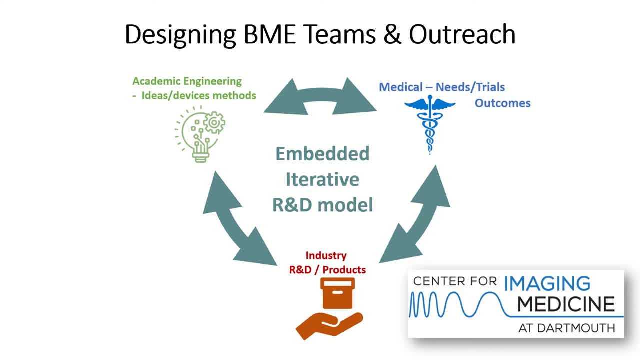 and that's all built into the medical center and that's what we've tried to do here at the Center for imaging medicine at Dartmouth, but it's this embedded model that really makes things work. so, as people are starting to think about what is the best way to improve their medical 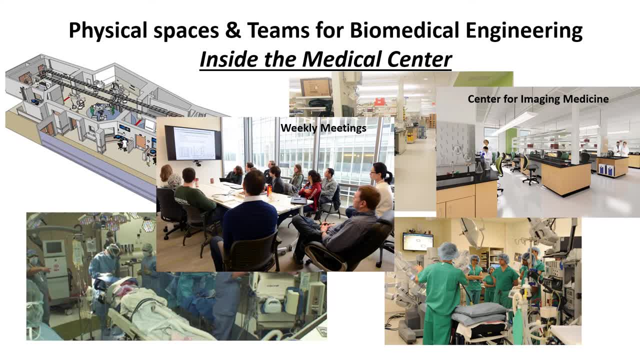 part of that creative space where you have biomedical engineers, academics and industry all in the same medical center. you need access to high technology, you need access to procedure based physicians need weekly meetings, you need biomedical engineering embedded in the medical center and that's what we've tried to do here at Dartmouth and a number of, of course, major medical